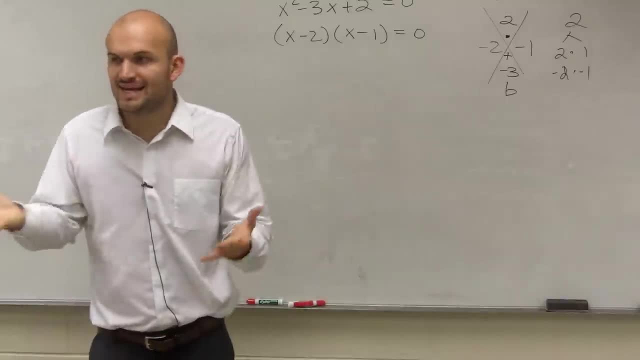 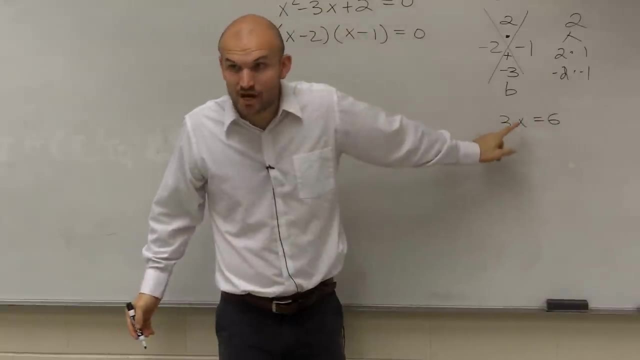 reason why you guys want to solve it by this way. right, because you guys, we can't solve it like this. You can't say 3x equals six. What do you do there? You get x by itself. right, That was easy. 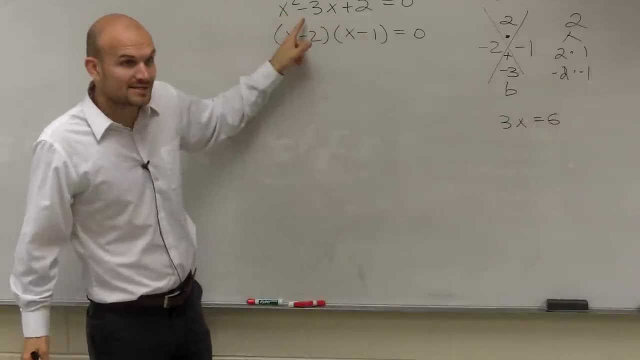 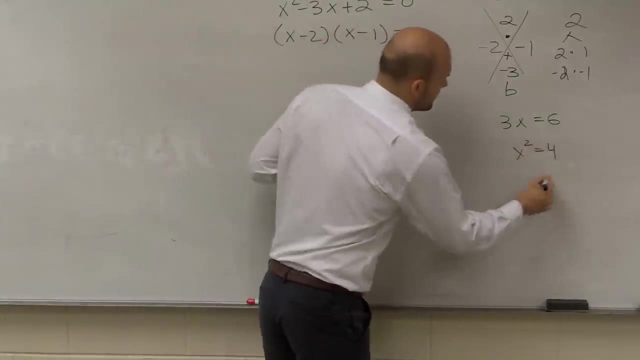 to get x by itself Here. it's hard to get x by itself. You get x by itself. You get x by itself Here. when we did this, what do we do here? We undid the square rooting right, But you can't undo. 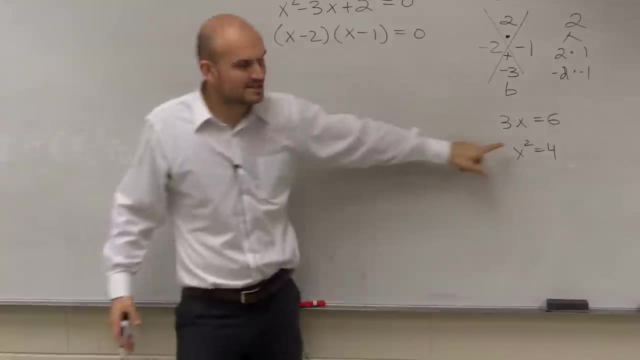 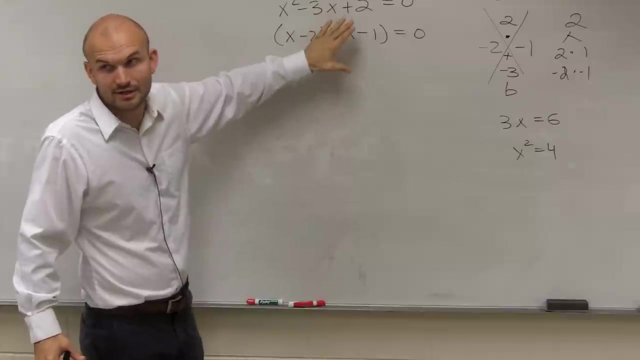 the square root, because then you're going to square root this x, So you just can't. so it's not as simple as these one and two step equations. So when you have a trinomial, or when you can create a looking trinomial, you have to break it up into your two factors. Now what I can do is: 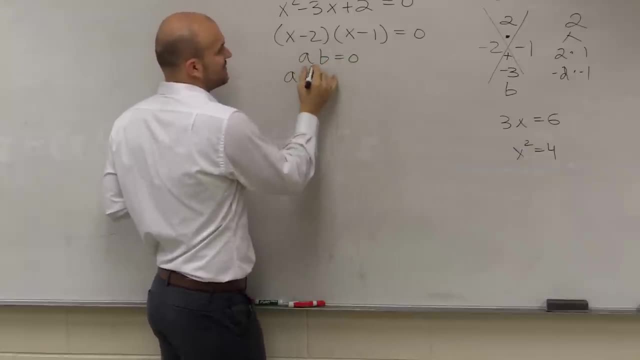 use my zero product property, Which states: if eight, if two numbers multiply to give you zero, or two factors multiply to give you zero, that means a equals zero or b equals zero. So therefore, Dustin, I can write x minus two. 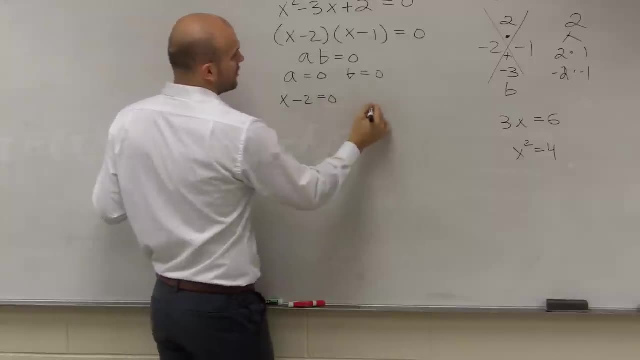 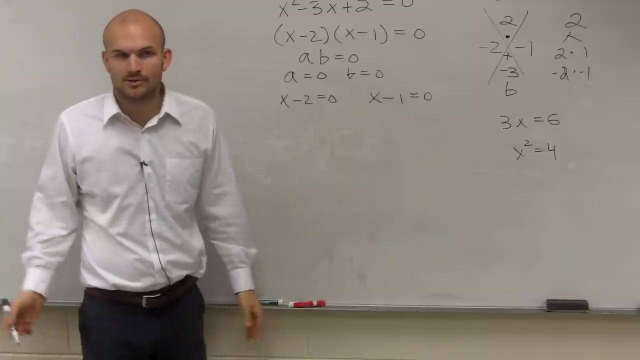 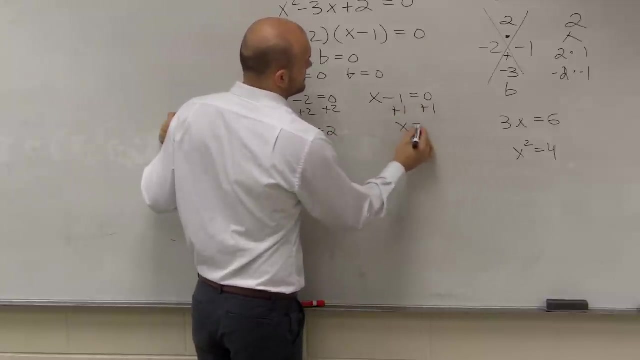 equals zero, or x minus one equals zero. Now can I solve each one of these equations separately? Yes, You can just say: add two to both sides, x equals two. Add one: x equals one. Dustin, does that make sense? 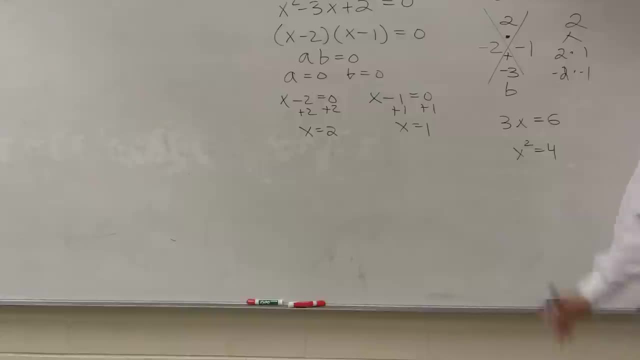 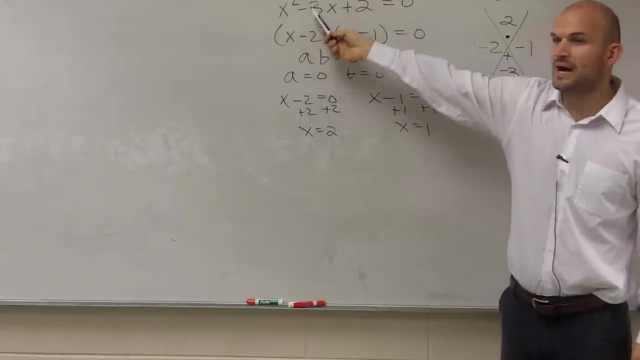 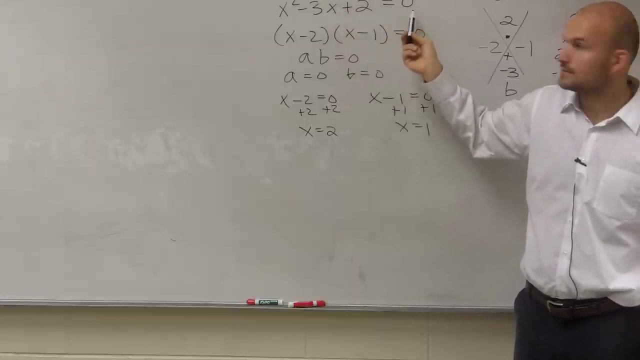 Huh, And that's your answer, Because plug in one into your solution. Remember, if it's a solution, that means it makes it true. right One squared is one minus three times one, which is negative. two. Negative two plus two is zero, right, Negative three. Negative three plus two is what? 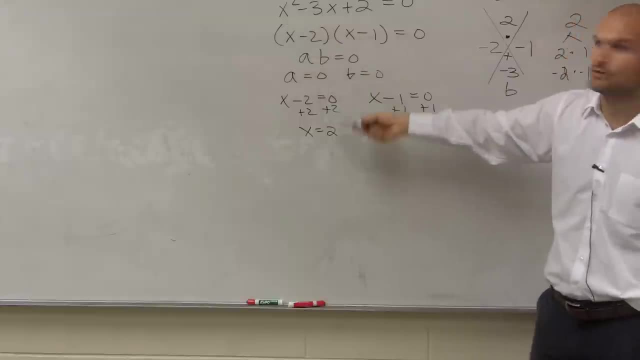 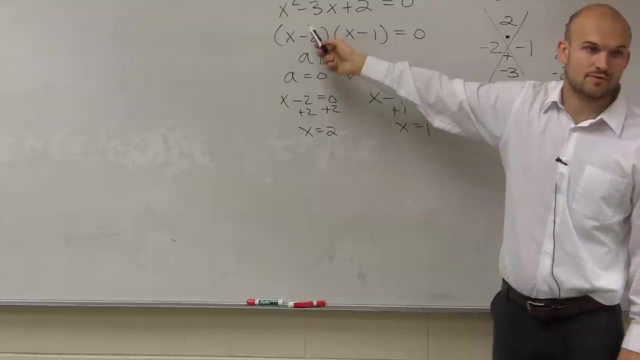 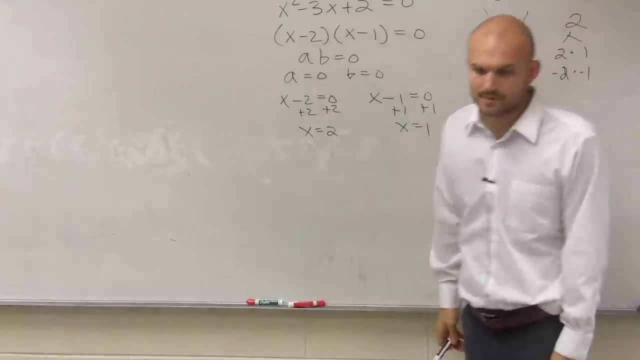 Negative one: One. Okay, Now let's do two. Two squared is four Negative three times two is negative six Four times negative. or four minus six is negative two Negative two plus two is zero. See how it works for both of them. There you go. Okay.